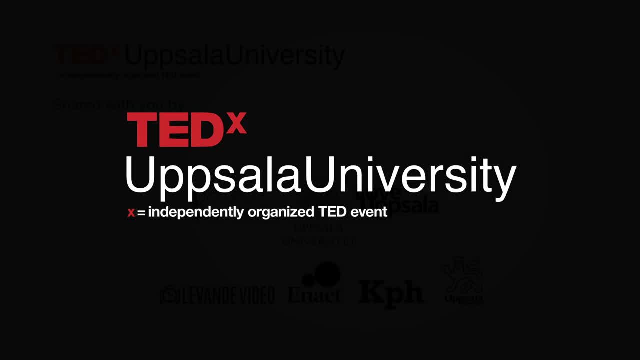 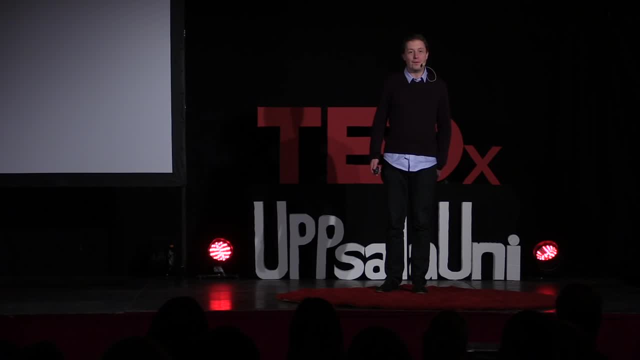 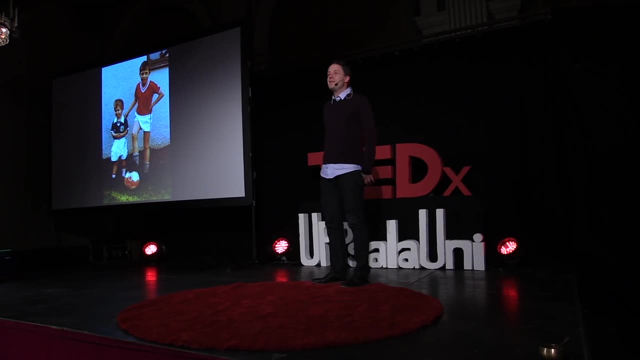 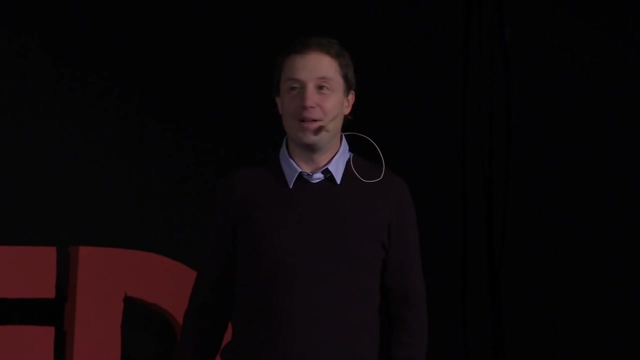 So when I was 10 years old, I absolutely loved football And more than that, I loved Liverpool Football Club. This is a picture of me when I was 10.. I'm the one with the Liverpool shirt, on the cute one with the Scotland strip. That's my little brother, Colin. Now, while 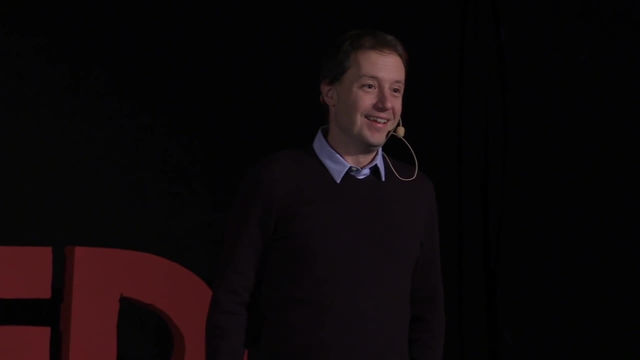 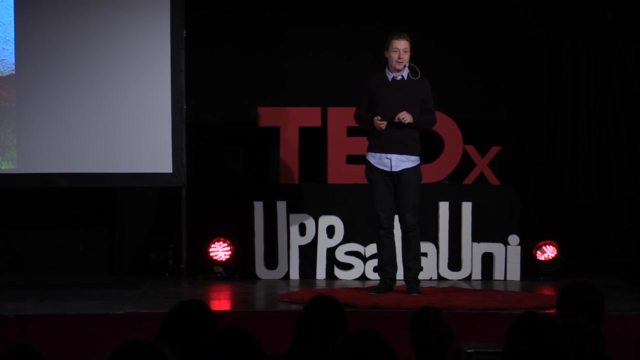 I loved football. I wasn't any good. You know that thing where you're in the school playground and two people have to pick teams to play against each other. Well, I was always the one who was picked last. But there were other things that I loved. when I was 10 years old, I really liked 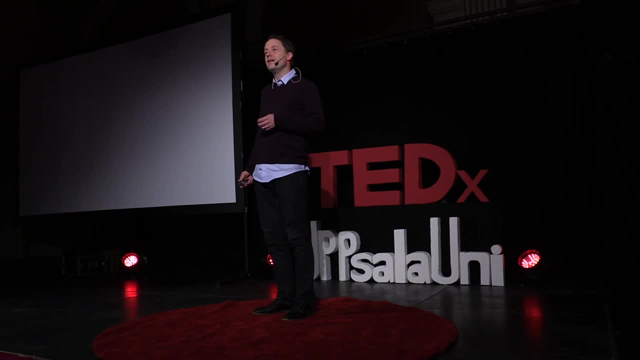 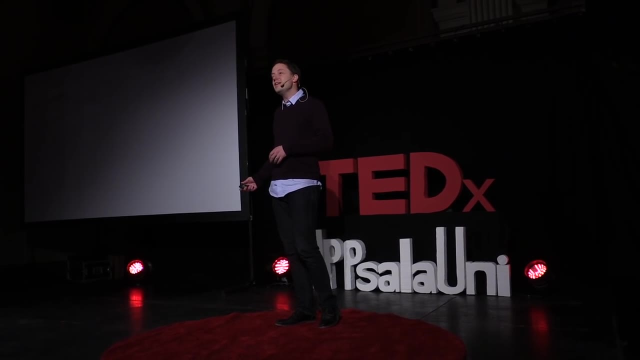 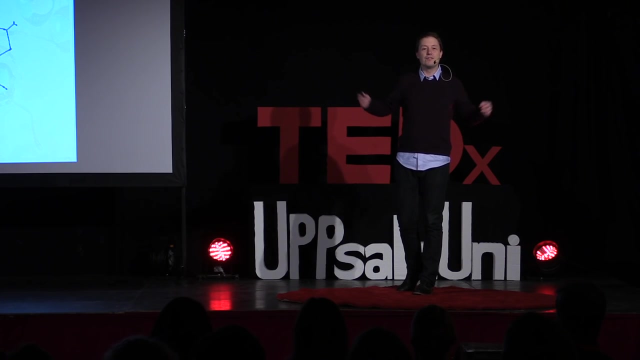 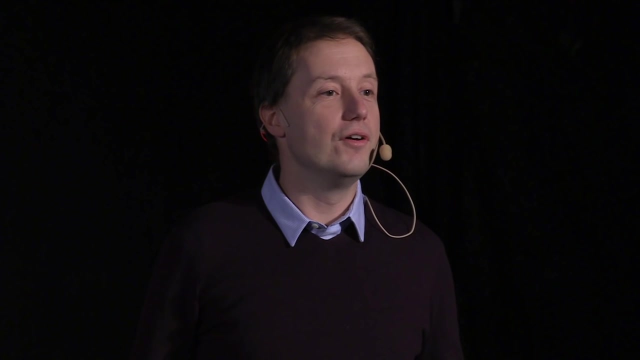 maths and I totally loved computers And those other two passions. they took me on a wonderful adventure. I studied the mathematics of ant trails, showing how these small animals can build massive transport networks. I looked at the algorithms behind how they organize their traffic and how they collect food. I studied the mathematics of fish schools, showing 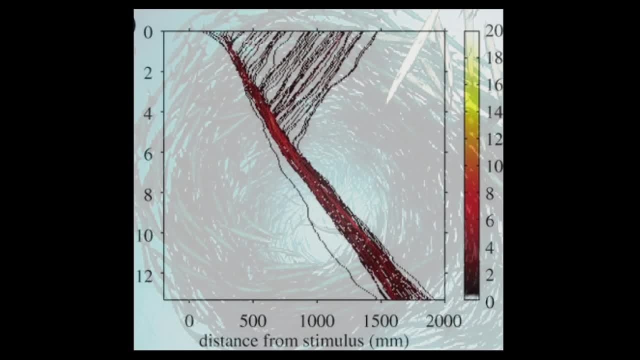 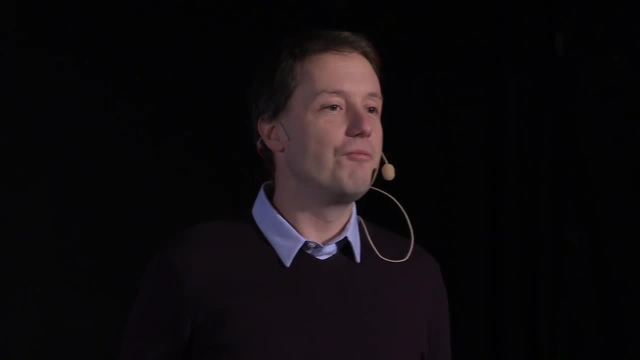 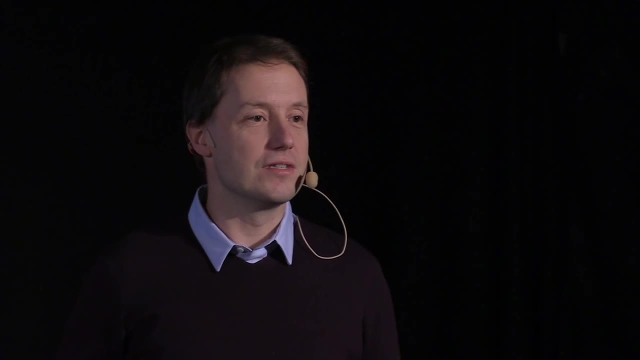 how they can escape as one from a predator, despite just interacting with a few nearby neighbors. I studied the mathematics of bird navigation: how they interact with each other, follow each other, how they produce consensus decisions, decide where they're going to fly together. 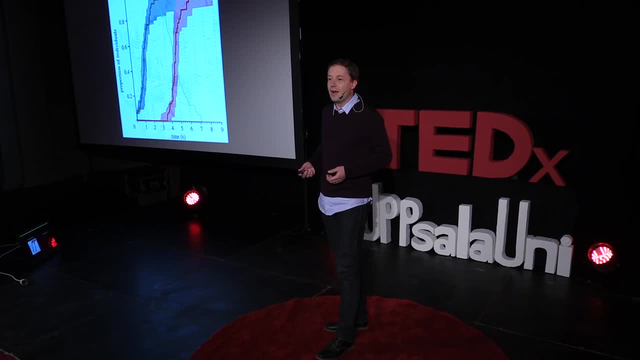 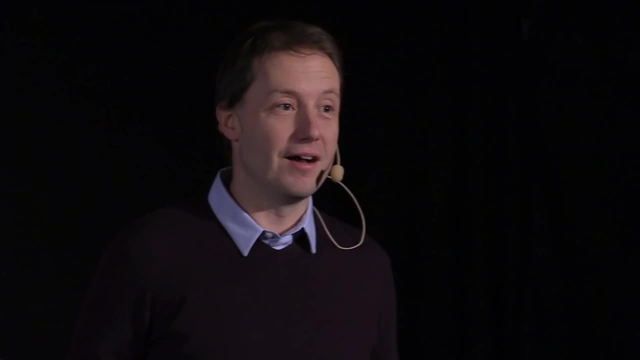 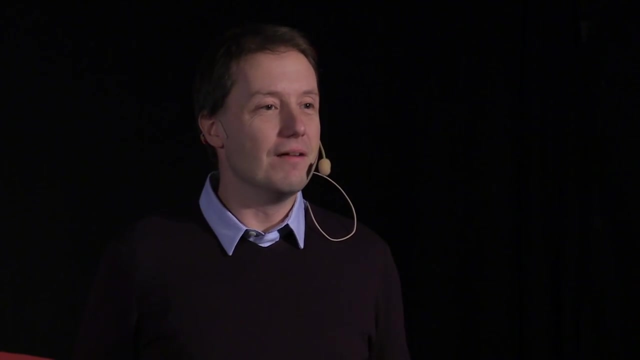 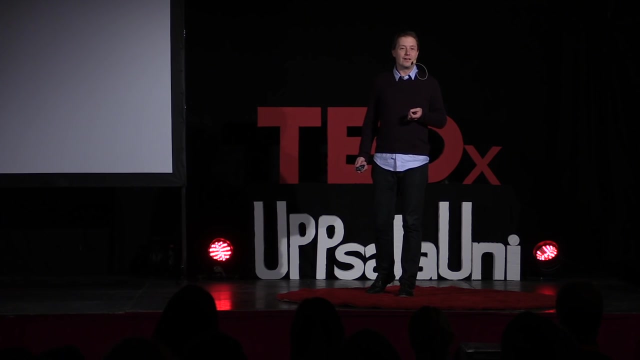 I studied our social behavior. I looked at how clapping was a contagion, how, when we coordinate our applause after a seminar or after a TED seminar like this, we can move together And coordinate in a very coordinated manner. And this mathematical journey I took has led. 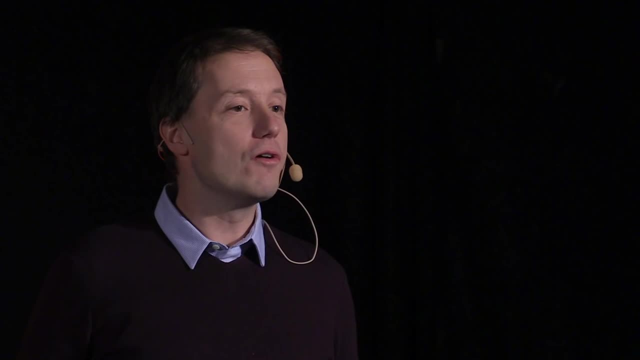 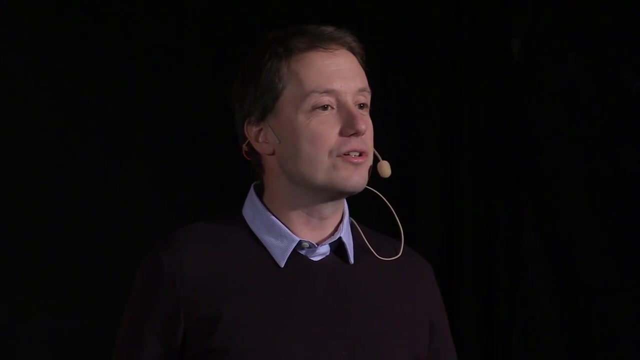 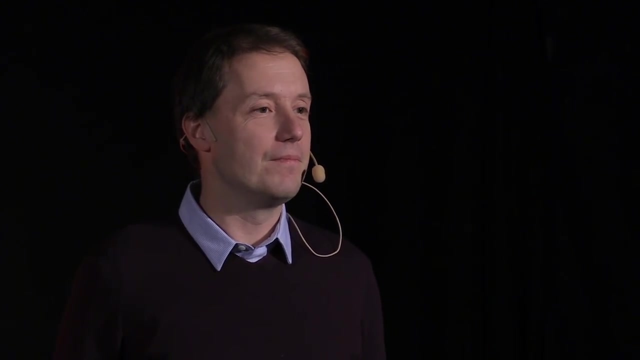 me all around the world to collaborate with lots of different researchers at different prestigious universities. I have the most amazing job. I get to talk to people about different systems and then I get to build mathematical models which help them understand these systems better. But the football, though. I never completely forgot about football. I never completely. 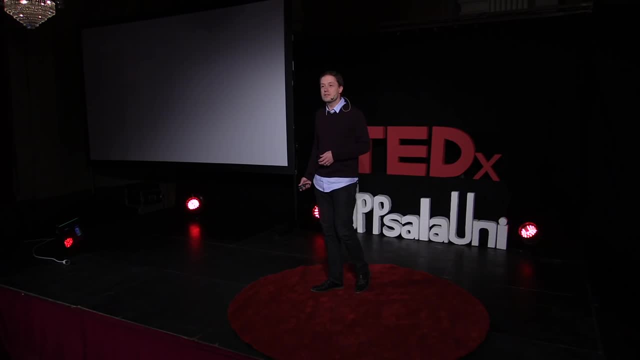 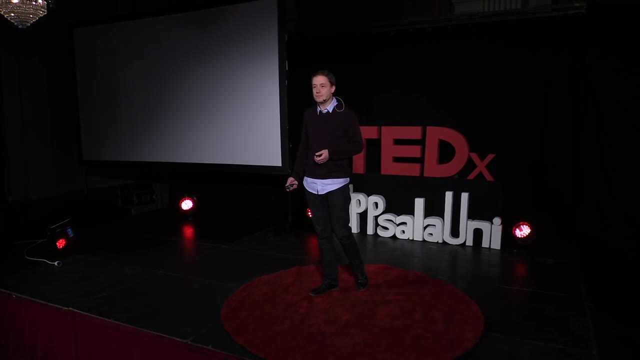 gave up on the football. I still played with friends, still badly. I watched it on television, I went to matches But I never really saw any connection between my interest in football and my interest in research. The friends I had who were interested in football well, 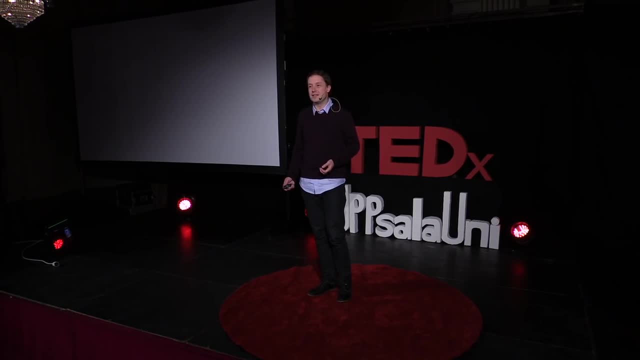 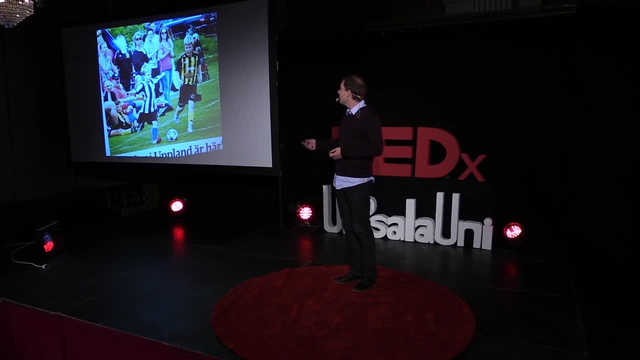 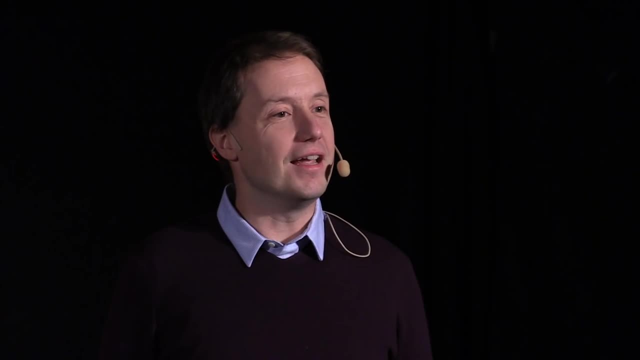 the first time I've ever done this. This is the first time I've ever done this. This is my son, Henry, when he was 9 years old. He's playing. this is a picture taken from the local newspaper. He's playing against boys twice his size. It turned out that Henry 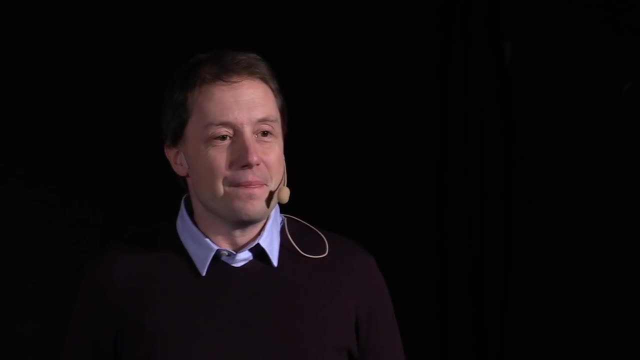 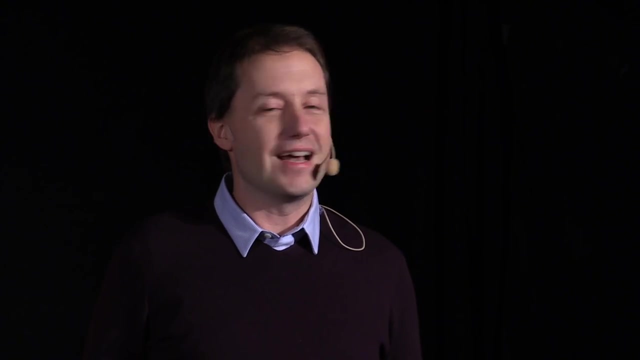 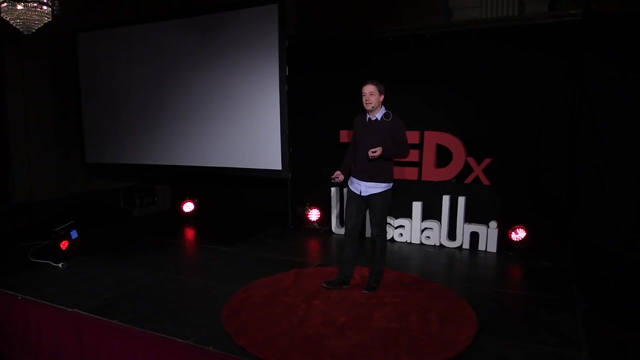 had the talent which I lacked, And so did lots of his friends, and I ended up with a bunch of other enthusiastic dads coaching Henry's team, Uppsala EF, And it was really then that I started to think again about: was there a coupling between mathematics and 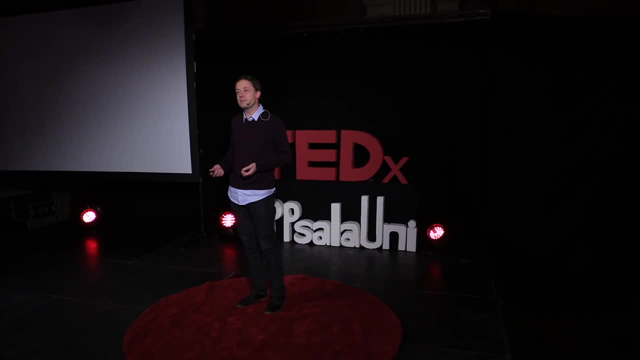 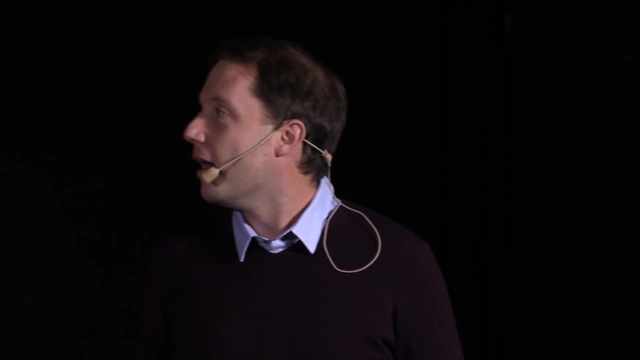 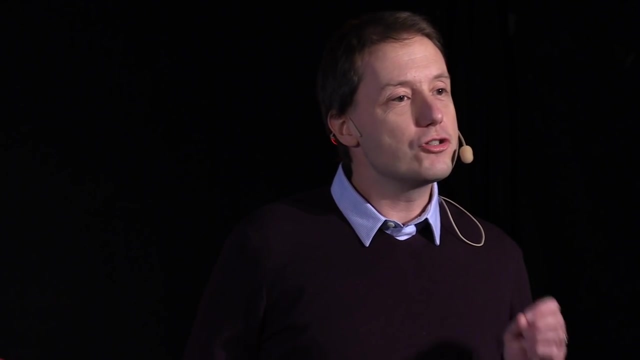 football. When I was training these players, I was trying to see if there was mathematics behind it, And I found a lot of mathematics in football. I started with randomness and last-minute changes of fortune. I worked out that about two-thirds of a football match. 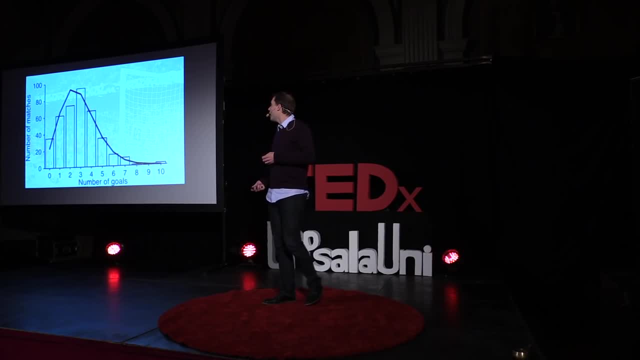 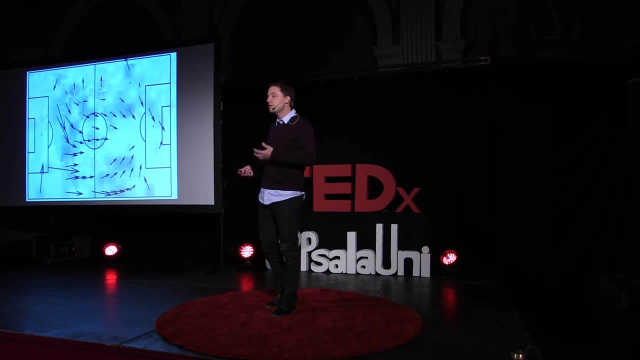 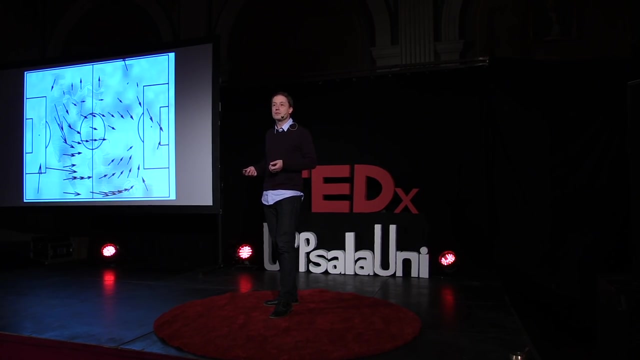 comes down to randomness. I looked at vector fields of passing of players and I could make player forecasts, just like we can make weather forecasts. I talked to Premier League scouts about how they could use these forecasts to pick the players that were best fit into. 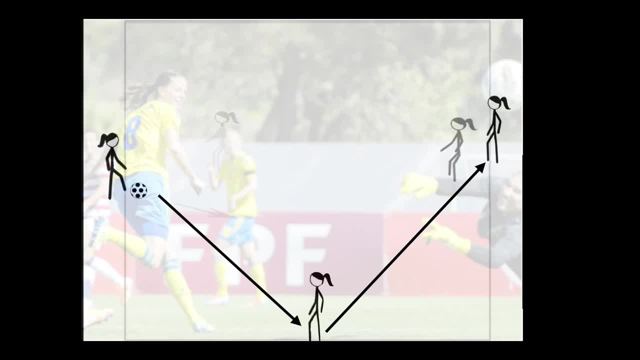 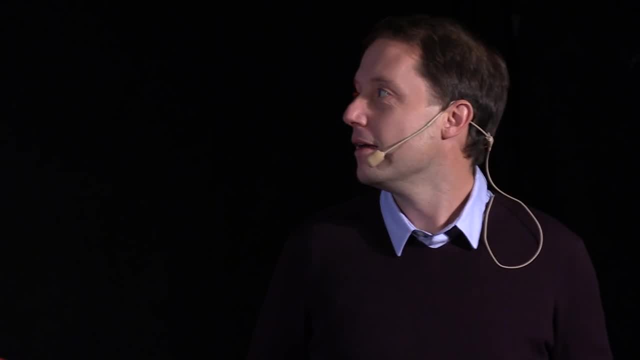 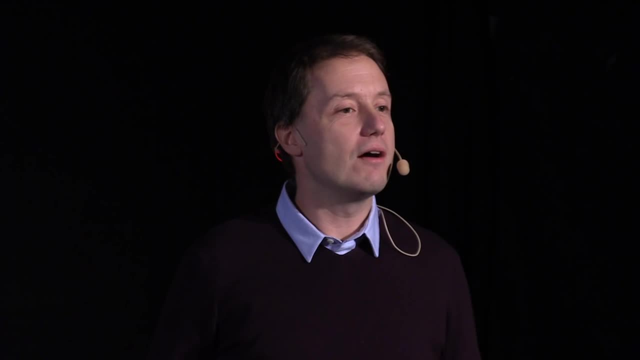 their team. I studied passing and positioning. I found out the best places to take a shot from and how to make a passing combination. I studied shots and goals in terms of statistics and probability and worked out who was the best striker in the world. 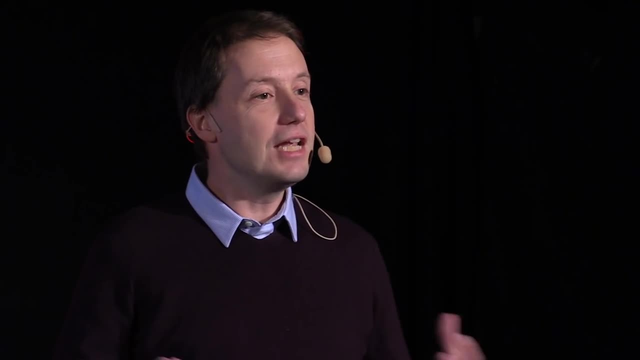 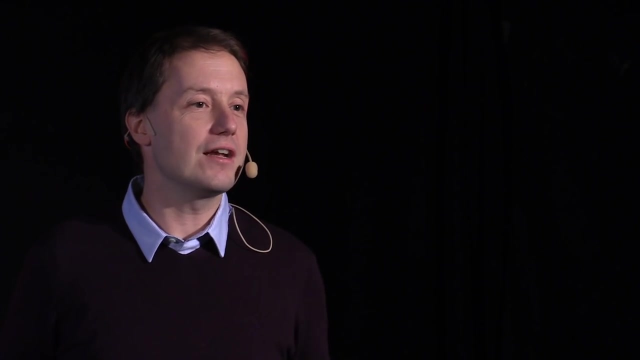 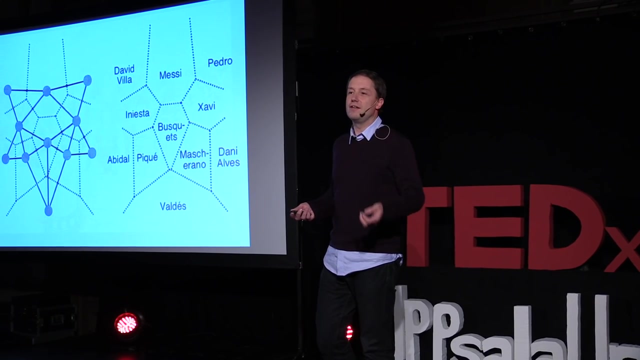 I looked at passing networks, how teams are connected together And managers use these passing networks to scout out the opposition, find which connections are most used and try and break them down. And I studied the geometry of the game. I worked out that Barcelona's 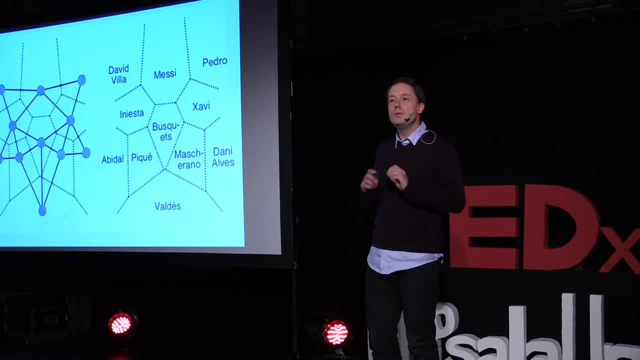 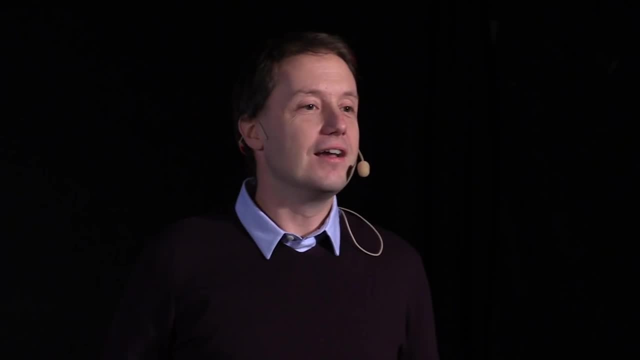 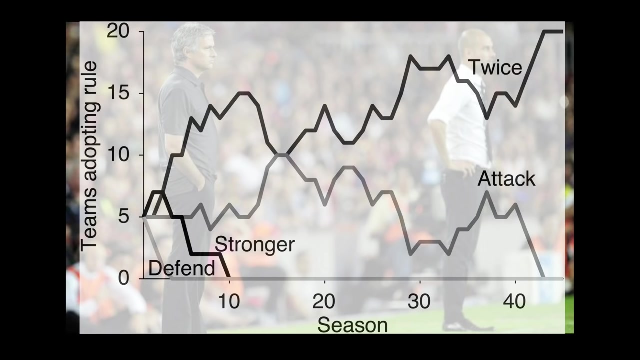 team of 2010-11 created the most beautiful geometry ever seen on a football pitch And I looked at strategy and game theory and how they could be used to explain the evolution- the constant changing evolution- of football strategies, And I even studied the 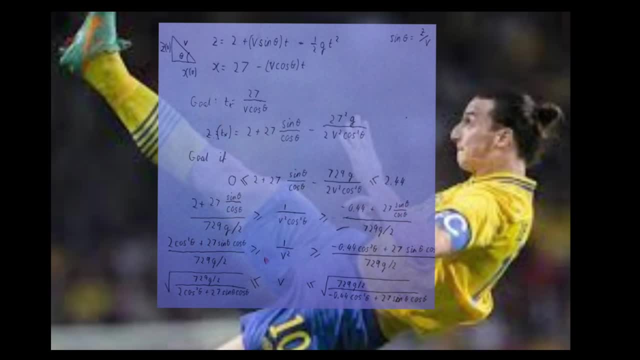 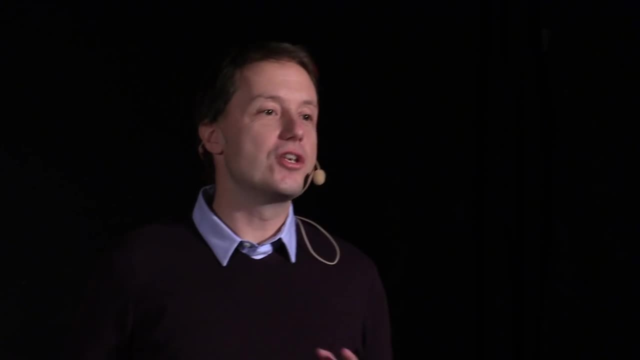 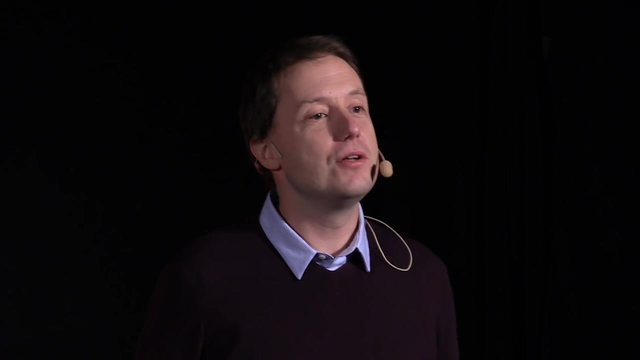 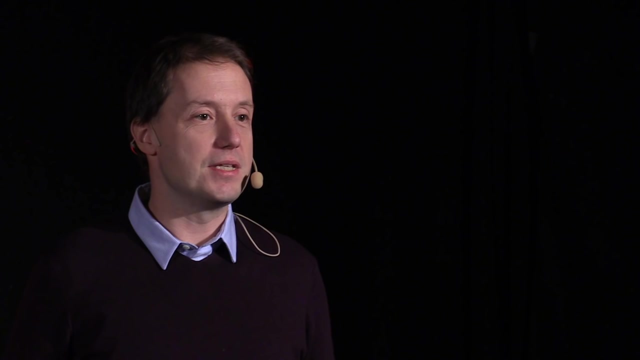 mathematics behind Zlatan Ibrahimovic's incredible bicycle kick against England. There is so much mathematics in football. Since I did all of these analyses, I've had this amazing opportunity to talk to Premier League scouts and analysts about how the game should be played. Most teams. 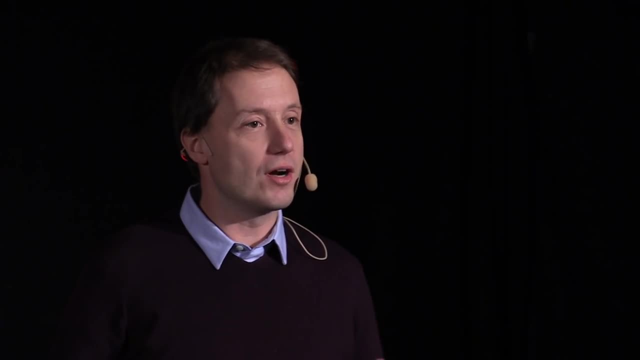 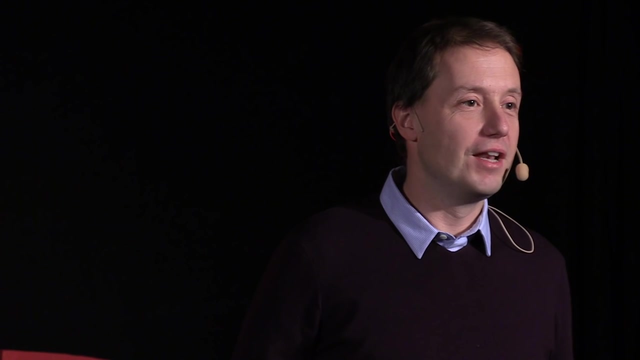 now have some form of mathematician who works for them and tries to work out how the team can play better together. One thing, though: I haven't yet been signed for Liverpool, And I thought I'd take this opportunity. Jürgen Klopp. 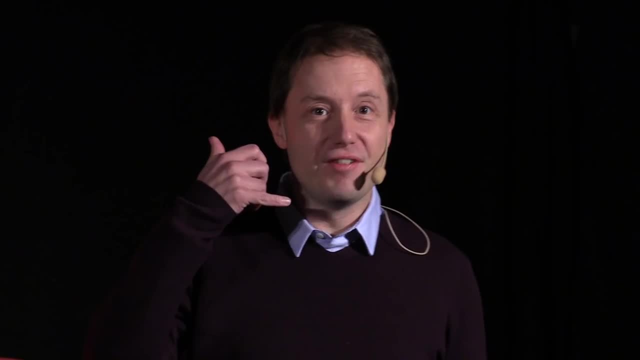 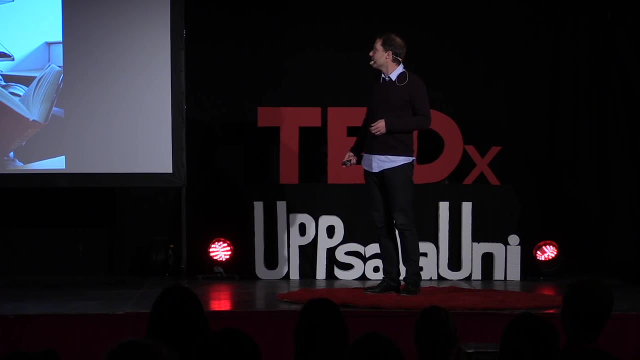 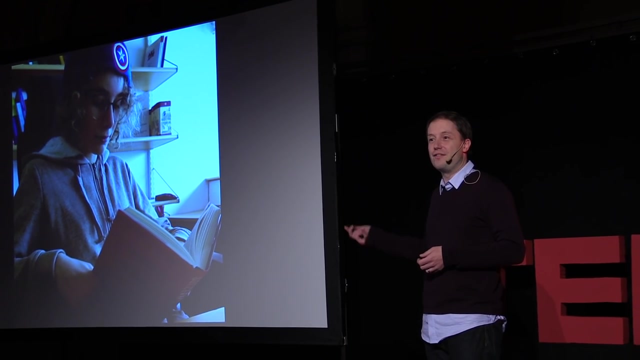 if you're watching, just give me a call, I'm available. This is my daughter, Elise. I finally, when I was going to give a TED talk, I finally got her to sit down and actually have a look at the book that I've written. 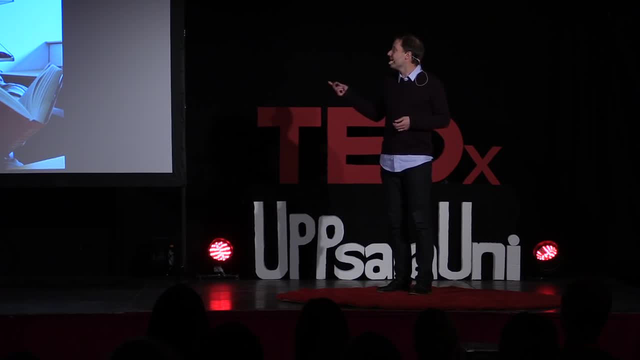 about mathematics and football. Elise is 13 years old and she thinks a lot about how the world works, just like I did when I was that age And when I was writing Soccermatics, when I was studying how mathematics and football were. 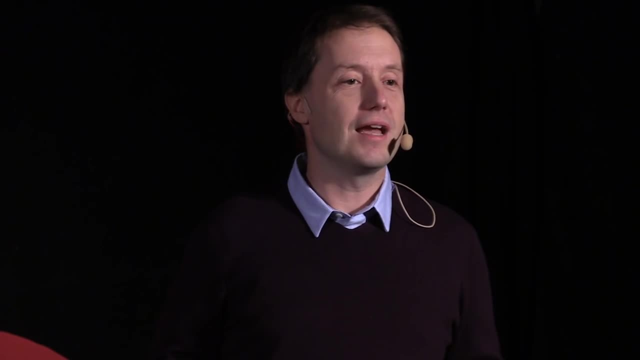 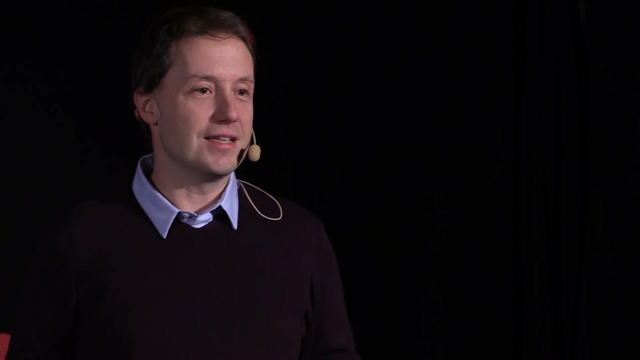 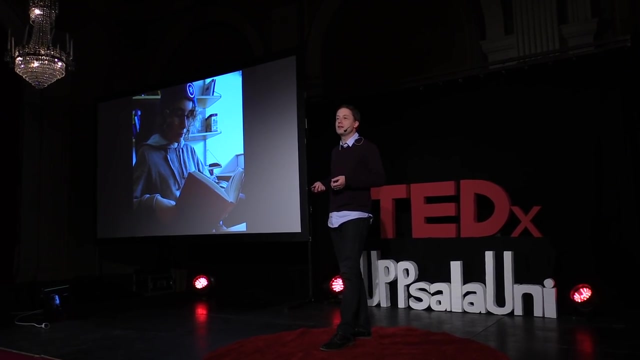 connected together. I'd often think about what I could communicate to her. Elise isn't interested in Barcelona's geometry or Ronaldo's shot statistics. What is it that I can tell her about the coupling between mathematics and football? The thing that I would. 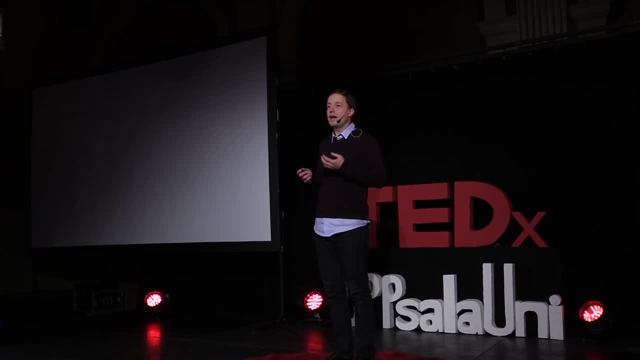 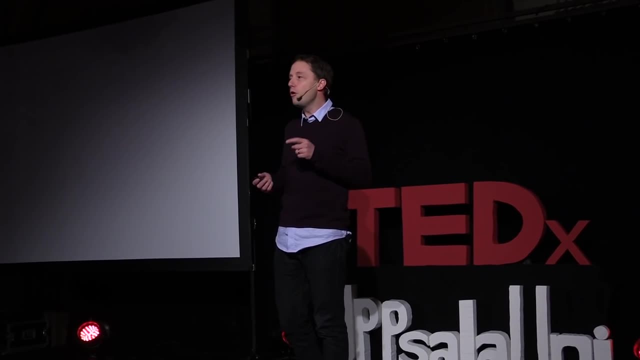 like to say to Elise and to Henry and to all of you, is that mathematics is not for some detached geniuses. It's not about picking you, you, you You're going to be in the best team and other people aren't in the team. Mathematics is. 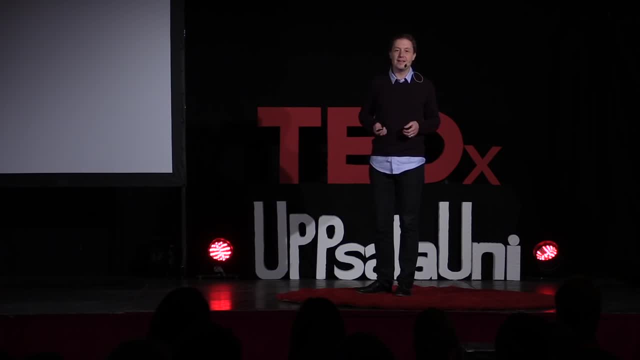 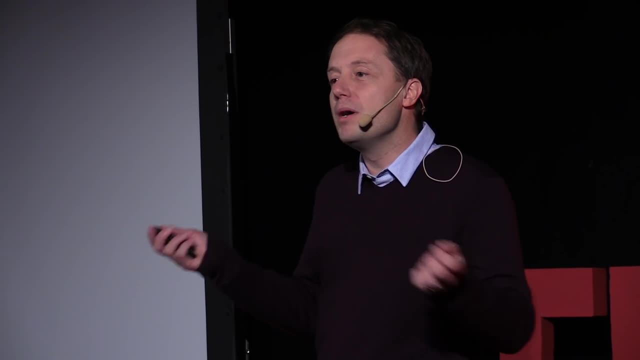 like a kickabout with friends. It's about getting stuck in. It's about getting dirty and enjoying yourself. It's about using your imagination. It's about using it's building up analogies between different parts of the world. Mathematics is something that 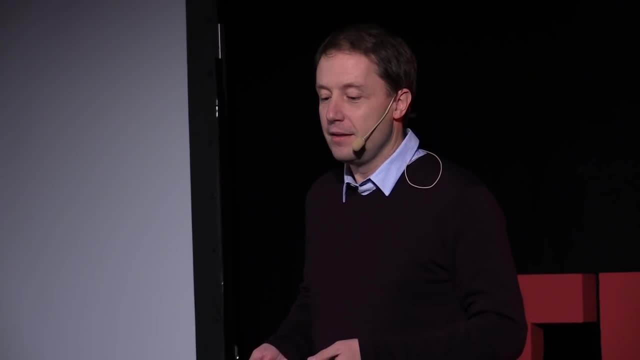 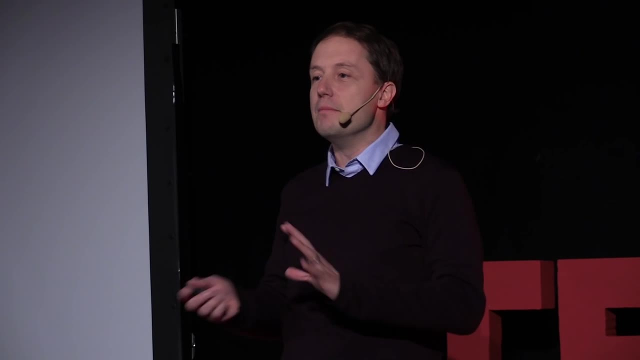 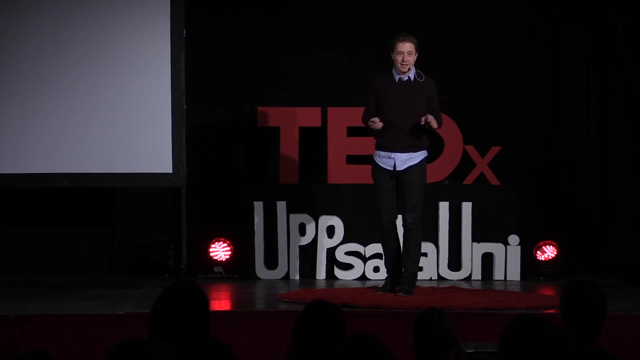 all of us can and should be doing Now. often at talks like this, you see someone like me waving their hands about saying mathematics is in everything, Mathematics is everywhere Way, And I have just done that and it is something I agree with. There is a lot. 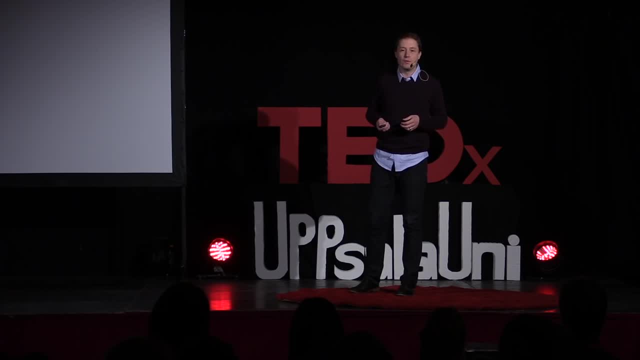 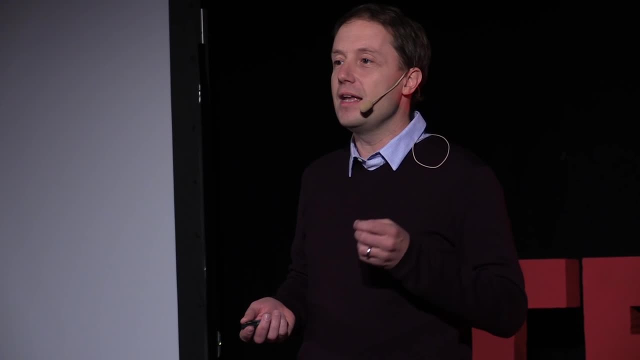 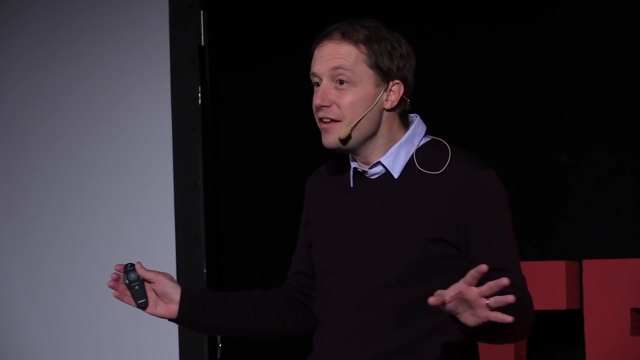 of mathematics in the world. I showed a lot of mathematics in football, But while there is mathematics in everything, it doesn't mean that mathematics is the answer to the meaning of life, the universe and everything. The answer isn't 42. It isn't any other number. 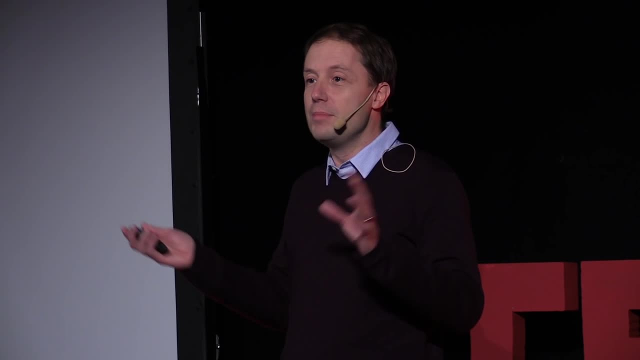 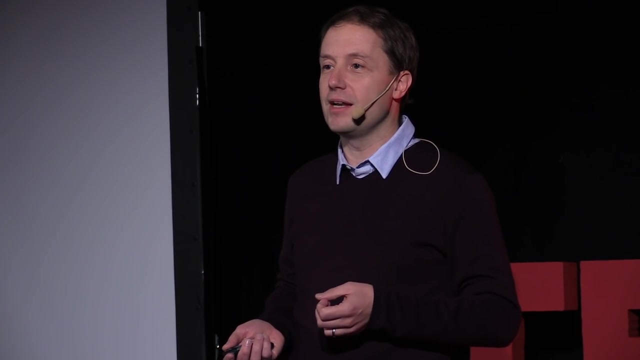 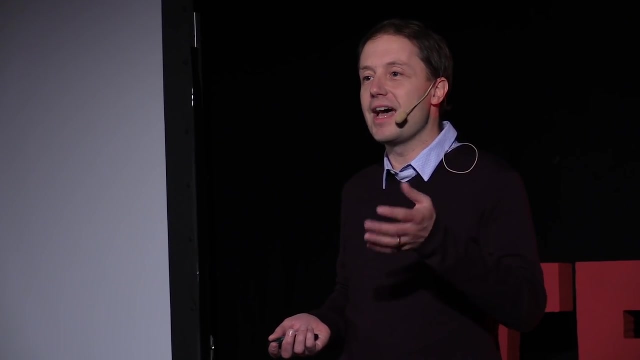 It isn't some complicated equation that nobody else understands. What I learnt from thinking about maths and football was a lot more modesty about my subject. So I can study Newton's equations as much as I want, but I'll never be able to do a Zlatan Ibrahimovic. 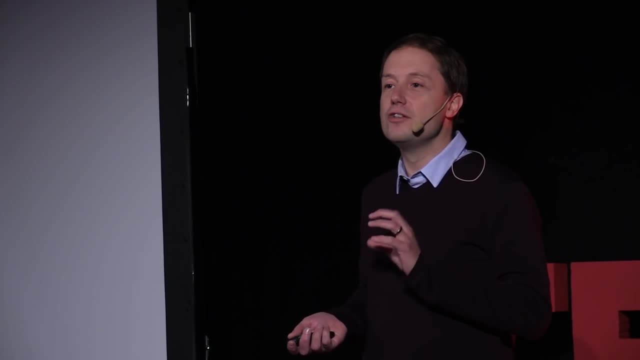 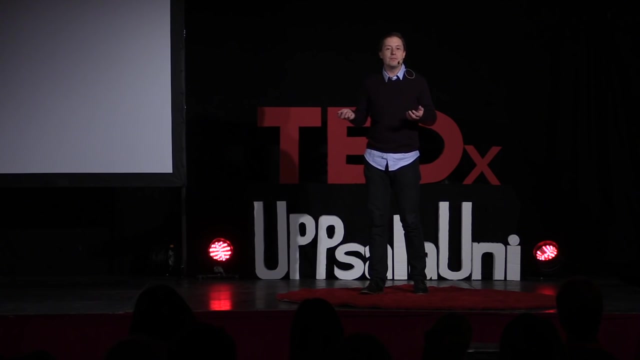 bicycle kick. I can study the geometry of the country of Barcelona, but I'll never be able to pass in the way those players can. I can study game theory and strategy, but I'll never be able to manage a team like Pia Sundhagen or Pep Guardiola. 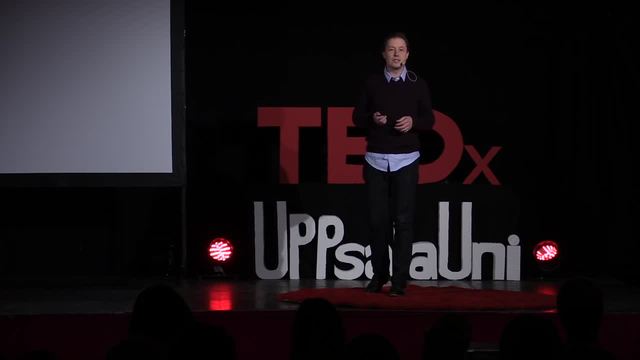 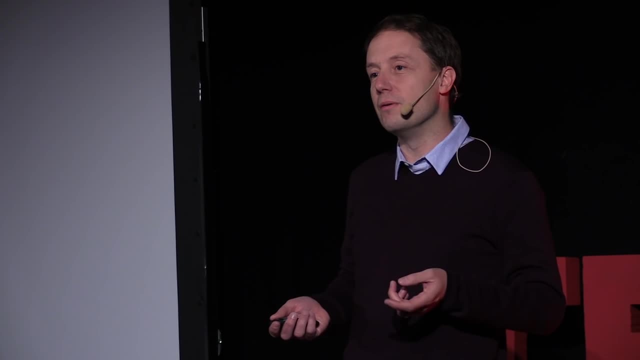 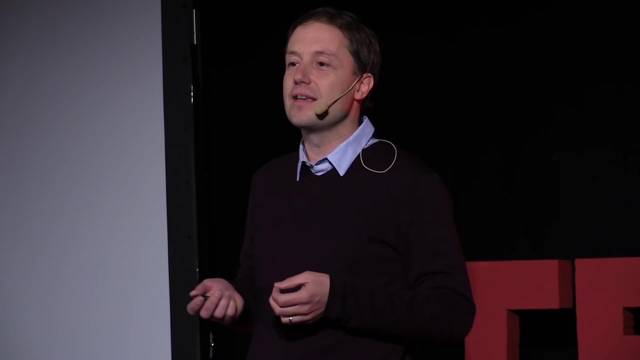 I can study as many fancy calculations, make lots of fancy calculations, but in the end I'll still be that boy, 10 years old, in the Liverpool strip, who can't play football and only has a small insight into this incredible complex. 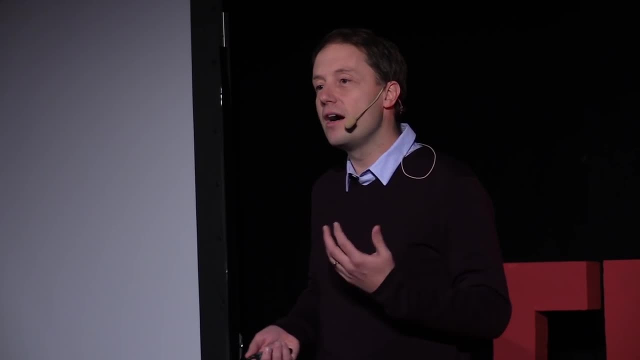 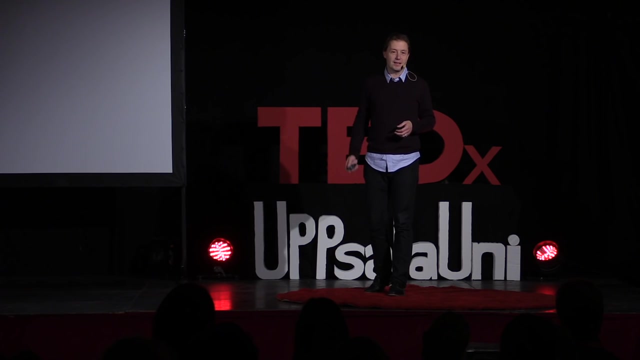 and complicated world we live in. Maths can't allow us to understand everything, not even close. There's lots of things in the world that we'll never understand. But what mathematics does give us? it gives us this edge. It gives us that little extra bit of 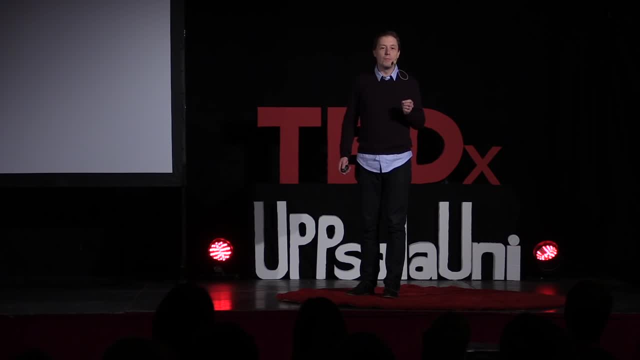 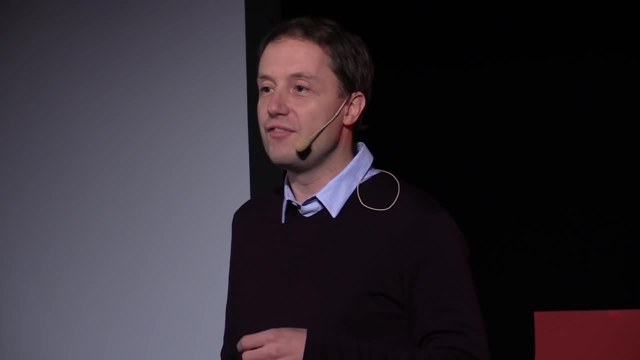 understanding. It allows us to win just a few more matches than we lose, And that is why mathematics is important to me, to you and every one of us. Thank you.